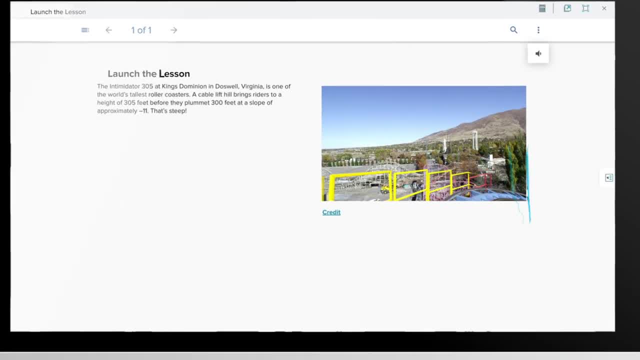 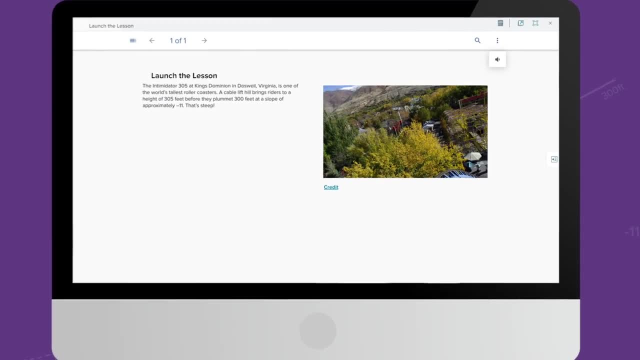 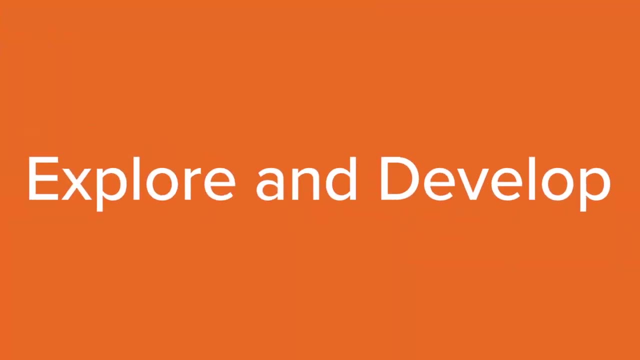 During the launch stage, class begins with a warm-up bell ringer and a launch the lesson activity to hook students' curiosity and guide them to become critical thinkers using the problem-solving strategies mathematicians use. Once these are completed, your class is now prepared to move on to the explore and develop stage of the lesson model. 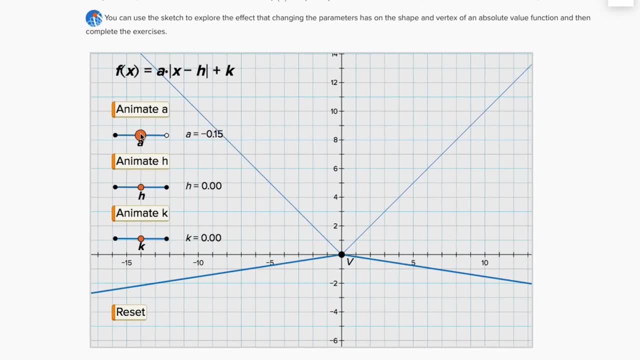 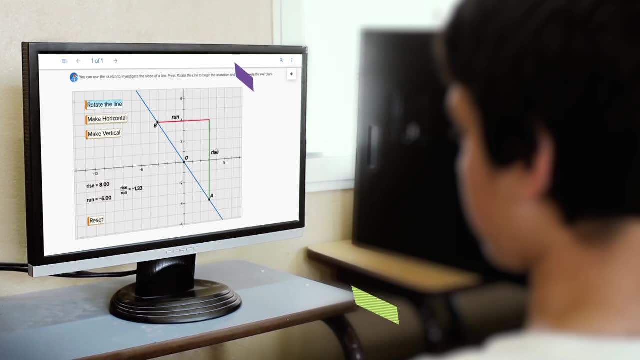 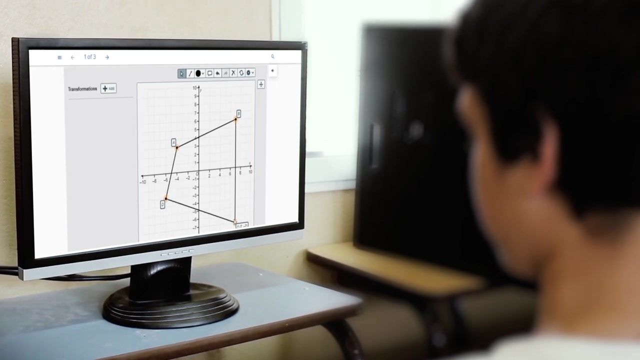 to uncover new concepts Here. most lessons within a module contain an explore activity which provides an opportunity to build conceptual understanding In the digital center. these activities and others contain a wealth of interactivity, including embedded web sketchpad and other e-tools so students can visualize the concepts they are learning In the digital center. these activities and others contain a wealth of interactivity, including embedded web sketchpad and other e-tools, so students can visualize the concepts they are learning In the digital center. these activities and others contain a wealth of. interactivity, including embedded web sketchpad and other e-tools, so students can visualize the concepts they are learning In the digital center. these activities and others contain a wealth of interactivity, including embedded web sketchpad and other e-tools, so students can visualize the 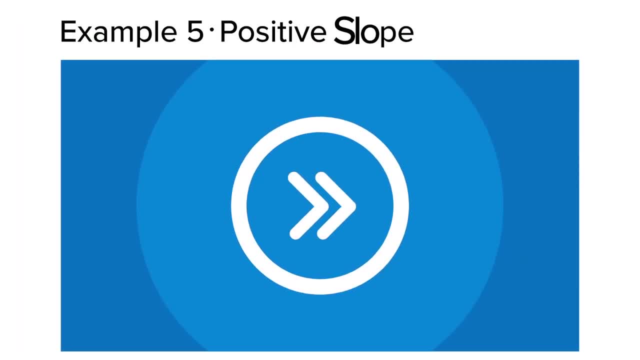 concepts they are learning In the digital center. these activities and others contain a wealth of interactivity, including embedded web sketchpad and other e-tools, so students can visualize the concepts they are learning, Also within the explore and develop stage of the lesson model. 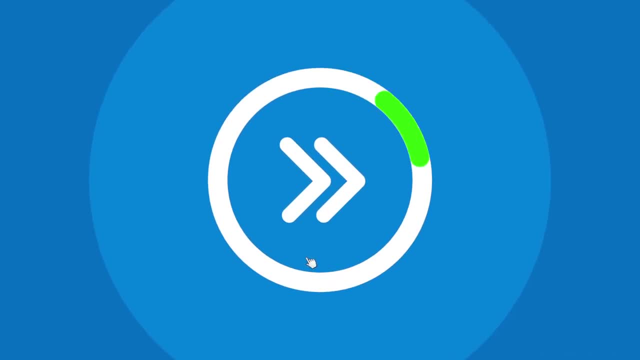 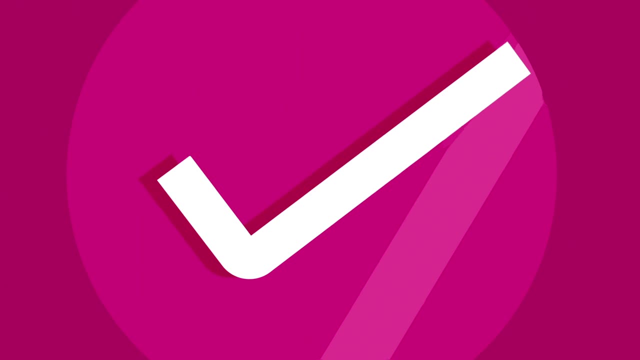 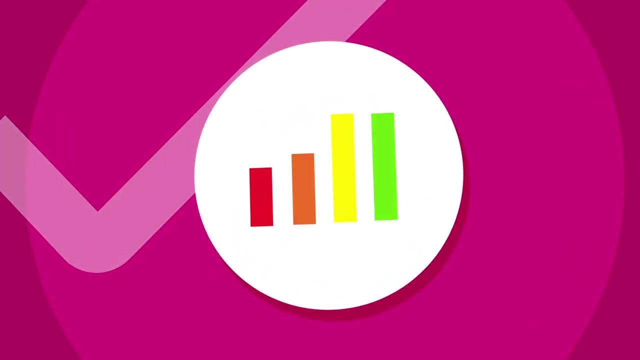 are multiple examples found in print and digital that are related to key lesson concepts. Once students complete examples, they are then followed by a check activity to assess student understanding and provide you an opportunity to adapt instruction, if necessary In digital, when activities with data. 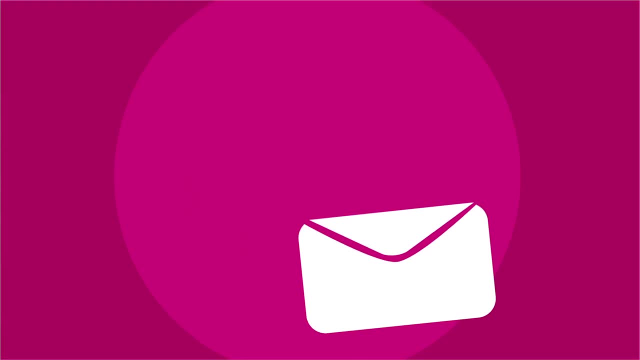 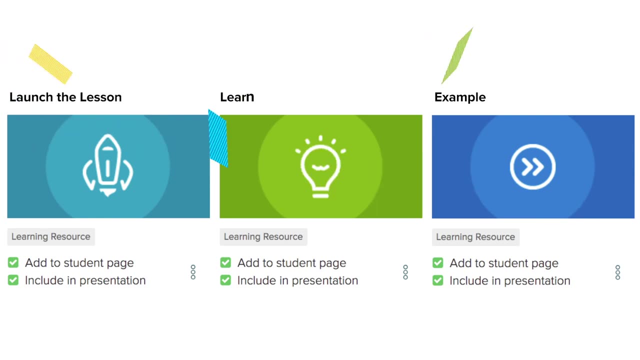 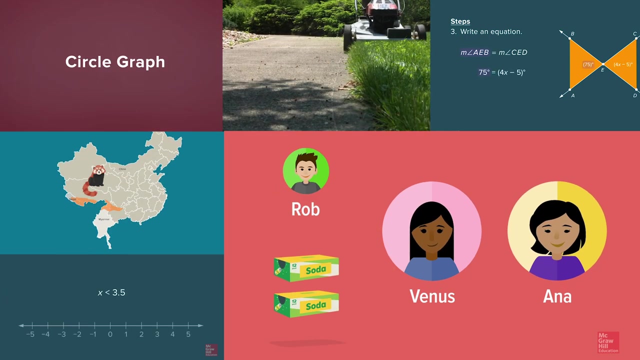 icons are assigned to students. data from that activity is sent to reports that provide valuable insight into your students' learning. You'll also find that within the launch, learn and example activities are videos and animations of real-world concepts to show the possibilities of math in real life. They're built into the resources right where they'll be most relevant. 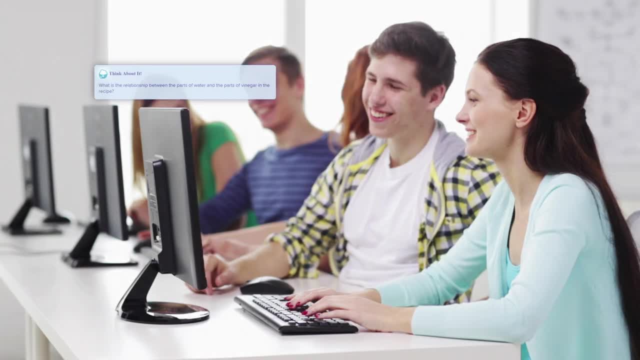 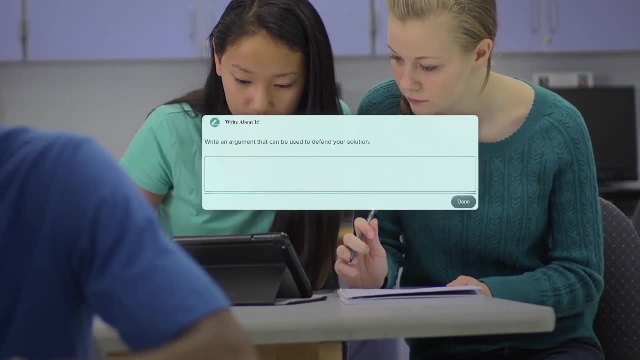 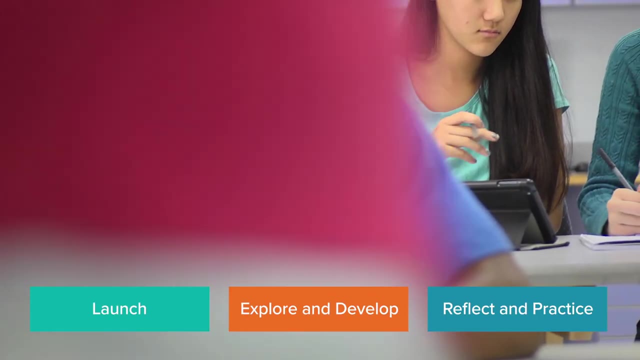 to your students. The examples in print and digital contain think-about-it and talk-about-it prompts, which are provided for mathematical discourse, and write-about-it prompts are built into the apply problems to help students justify their thinking. After students deepen their understanding in the explore and develop stage, they then move on to the reflect and 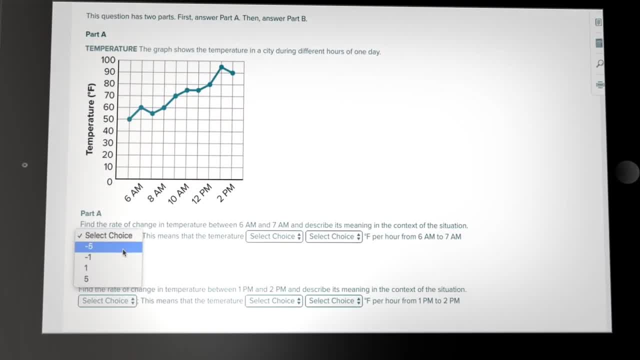 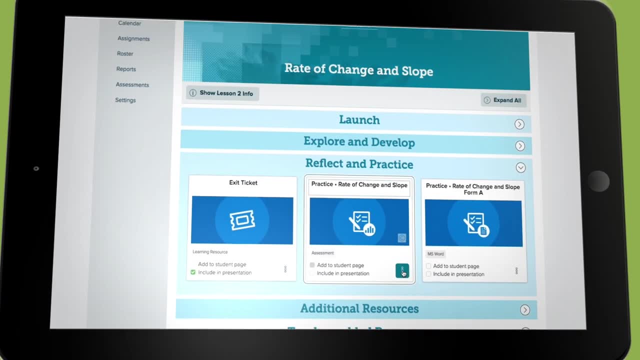 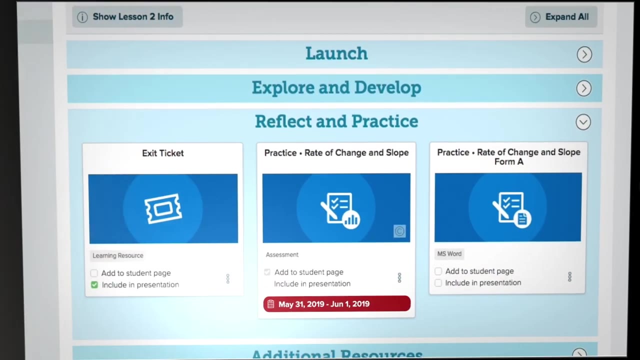 practice stage of the lesson model. Here teachers can have students work on the exit ticket to convey what they understand, followed by practice exercises that can be completed in print or digital where they can easily be assigned as homework. All these resource tiles in your